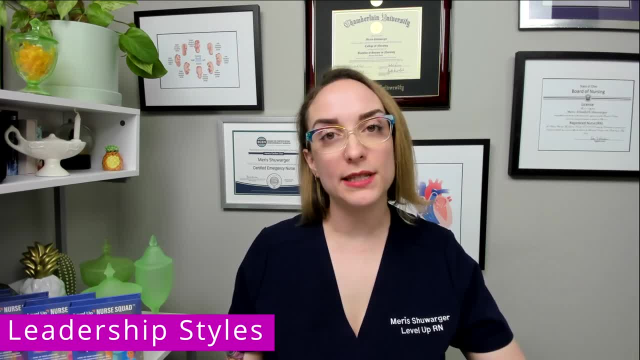 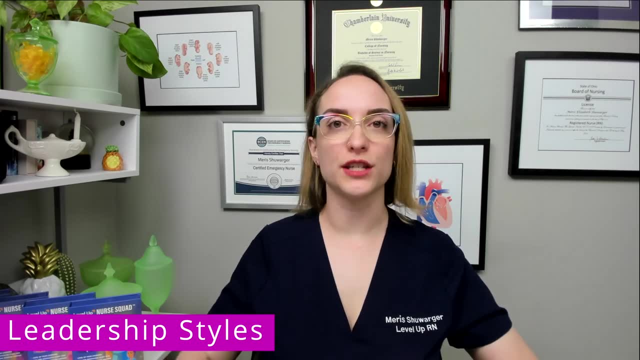 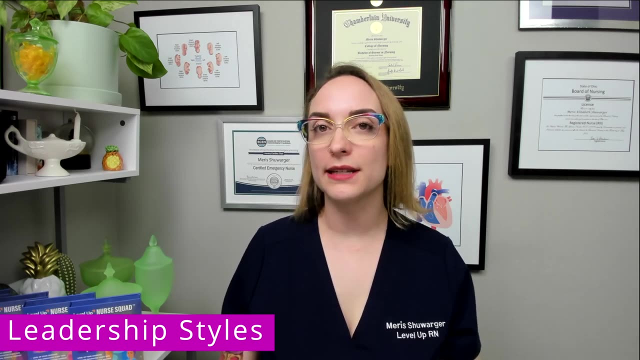 So this is useful during emergency situations. So think of like a mass casualty event. Somebody has to step in, take charge, give directions. This isn't a time to collaborate and have a sharing of ideas. It's an emergency. So this is good for emergency situations. It's not an ideal leadership. 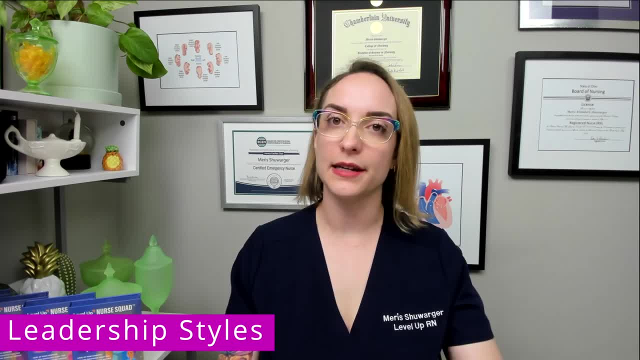 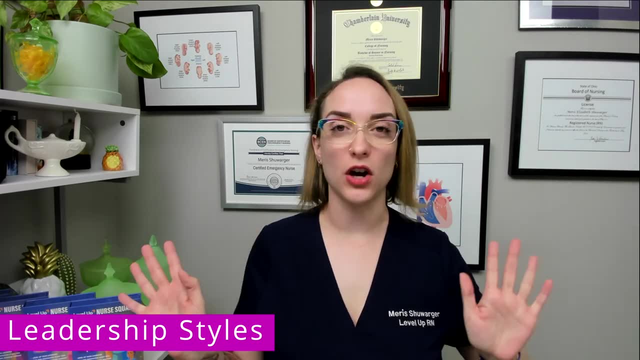 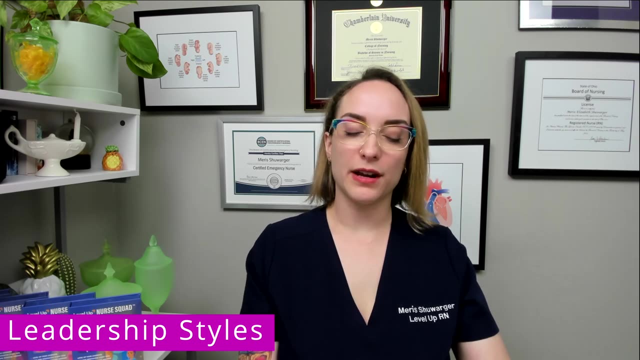 style for, like your everyday unit management, for instance. Now moving on to laissez-faire. When we think of laissez-faire, this essentially in French means hands-off. So this is the leader who kind of just lets people lead themselves. They're going to let the team. 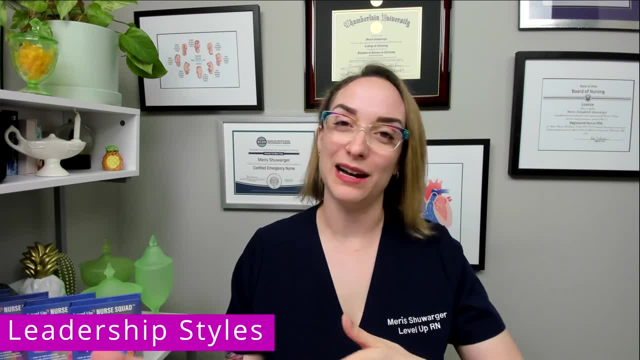 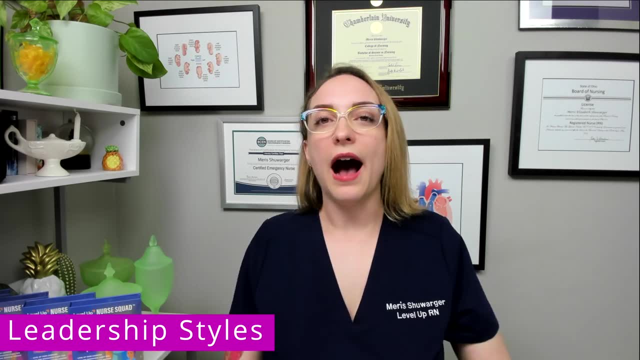 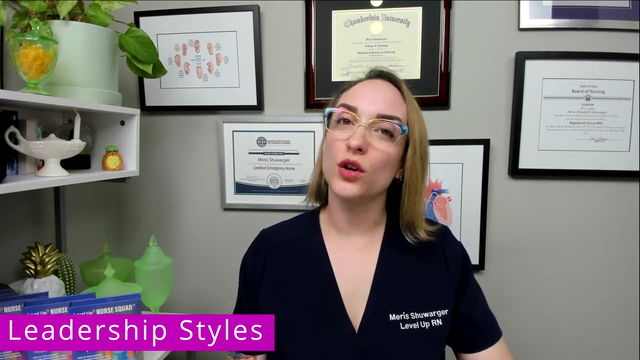 make decisions for themselves, And this might sound nice, but it leads to low productivity and frustration because there's no actual leadership going on. So it relies on the team members to make those decisions for themselves- Again, not ideal. And we do have a cool chicken hint here to help you remember that laissez-faire is lazy. So if you 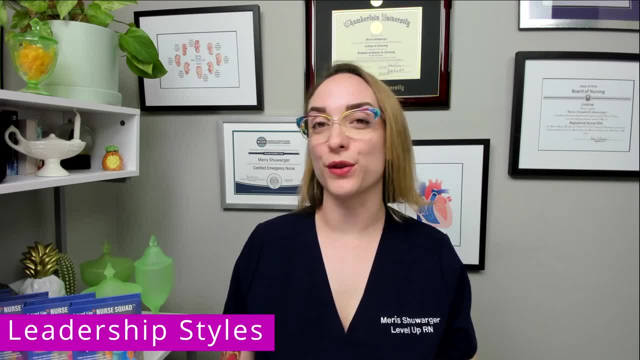 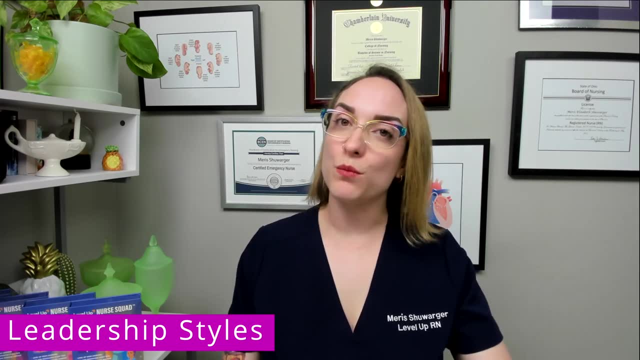 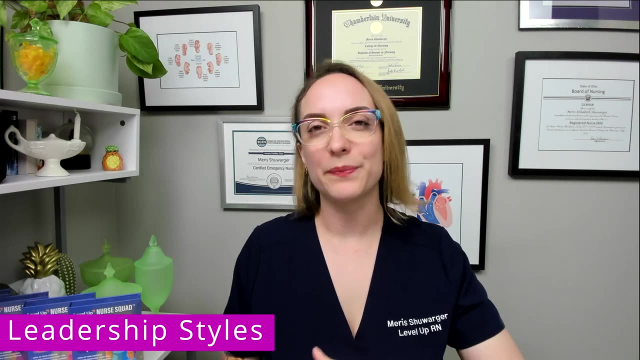 think of that when you are taking your nursing school exams or thinking about leadership styles. laissez-faire is lazy, Now democratic. This is where the leader and the team work together towards the goals and outcomes. It promotes group satisfaction, but it may slow decision making. 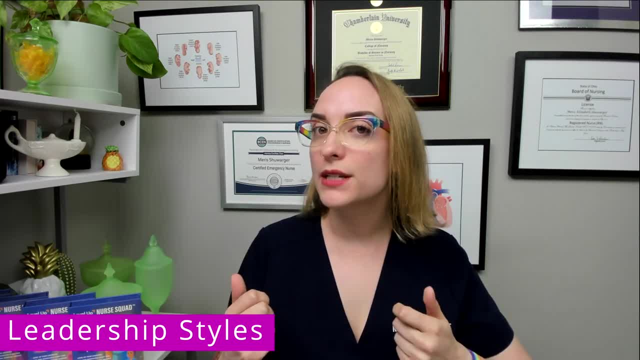 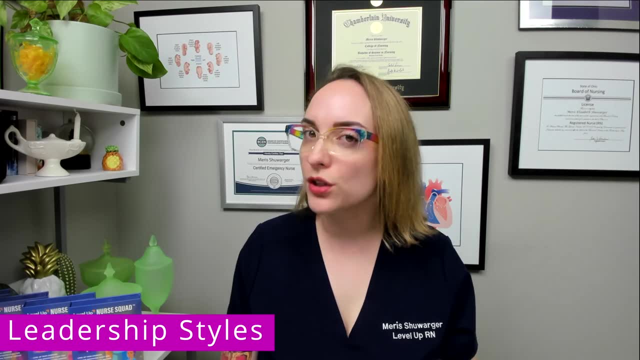 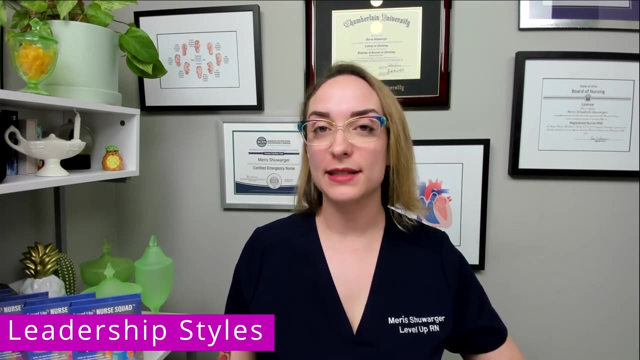 Again, if we are getting everybody's input, it's going to slow things down. It's not that this isn't necessarily a good leadership style, it's just a slow one. So keep that in mind. And then we have transactional. Now, with transactional, it is what it sounds like. I. 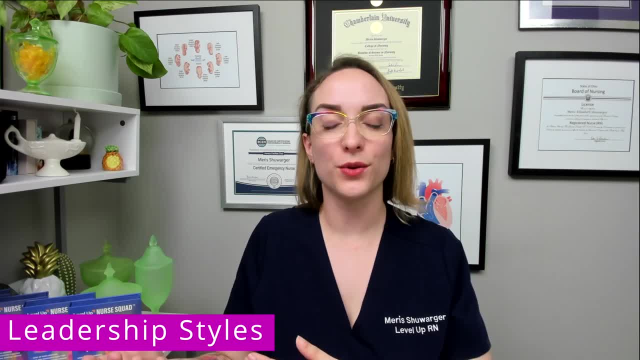 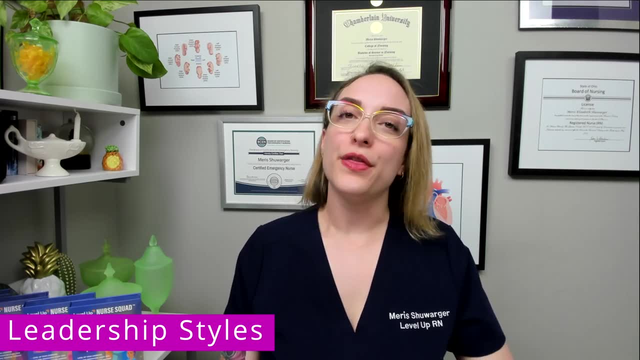 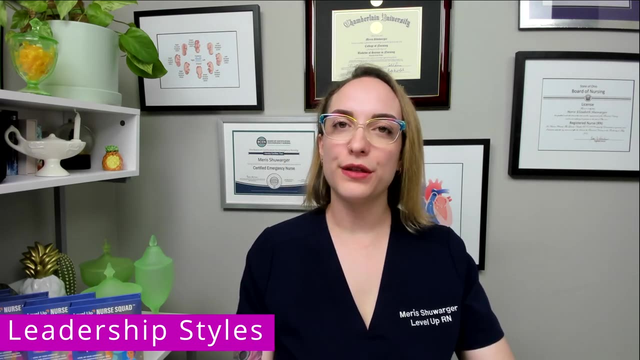 want you to think of a transaction Like when you go to the store: if I give you money, you give me a thing, right, That's the transaction. With transactional leadership, there is going to be a reward in exchange for tasks being done. Now, sometimes this might be a good thing Sometimes. 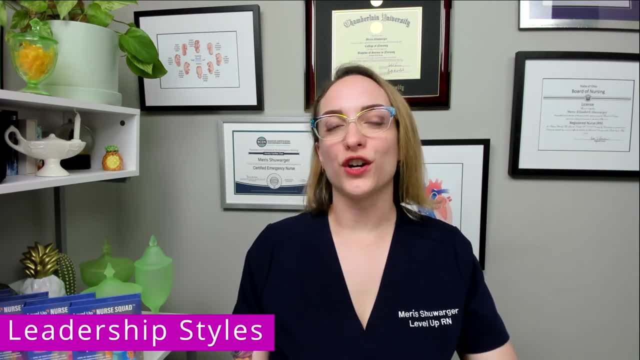 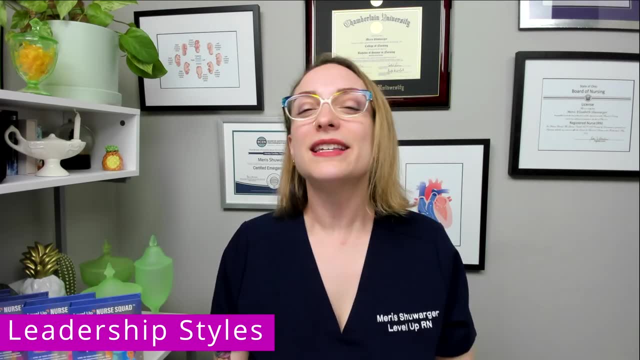 it's a nice, you know motivating factor, Like when you're, you know, the person who gets the most positive patient comments gets a pizza party or you know whatever. Sometimes that can be a good thing, But again, we don't want to necessarily always be motivating people with extrinsic. 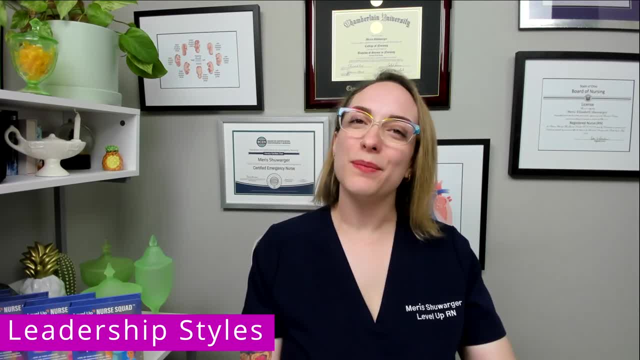 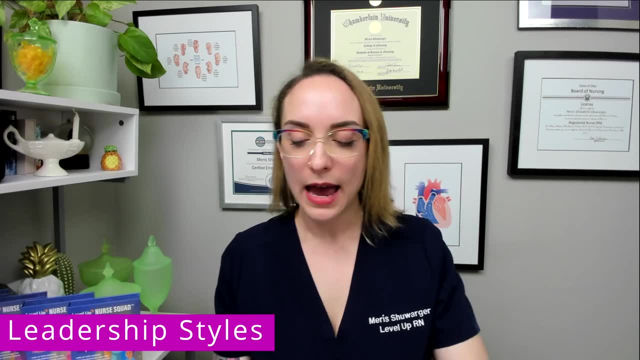 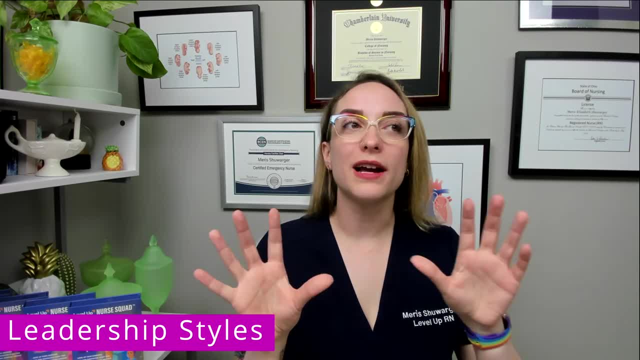 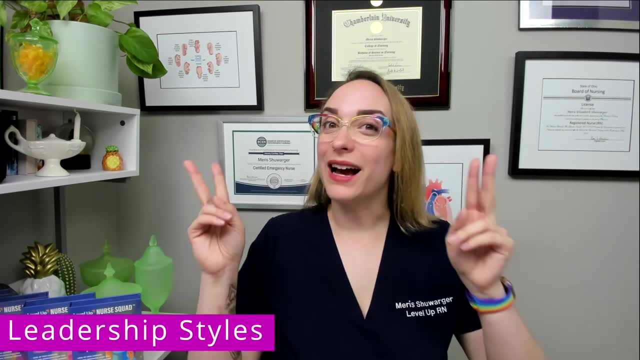 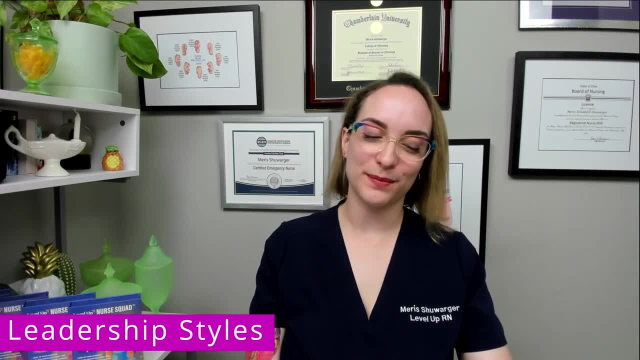 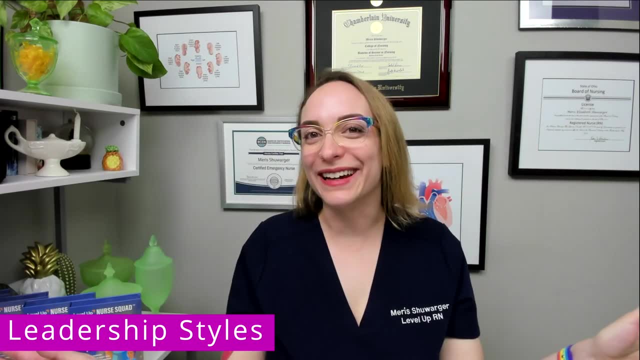 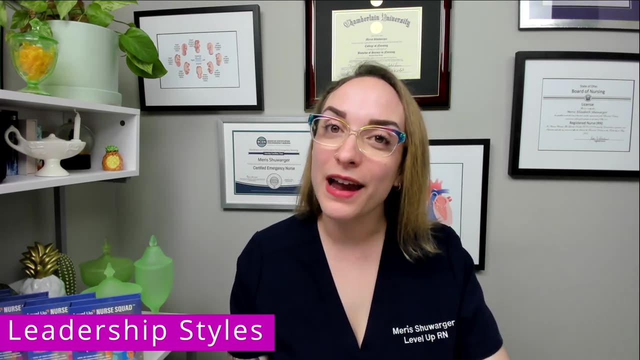 ideal leadership style. The ideal leadership style is going to be transformational. So we're not just doing a transaction, We are transforming the people beneath us with our amazing leadership skills. okay, So transformational. this promotes teamwork and shared decision-making. 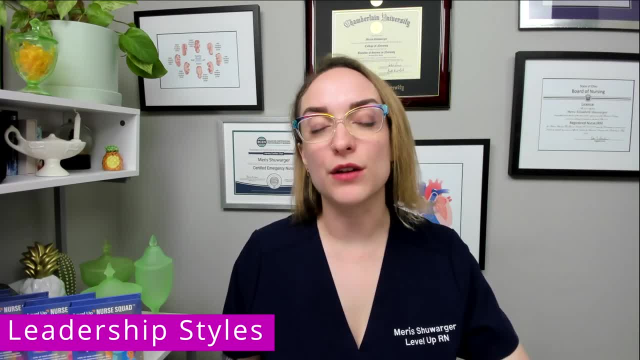 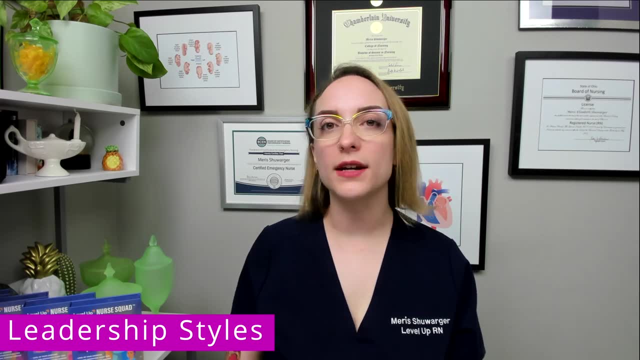 And the leader is going to be seen as trustworthy and respected. Again, this is the ideal style. So this is. you know, the leader is strong, They're making strong decisions, but they are considering input from the team. When I think of transformational, I often think of like a unit. 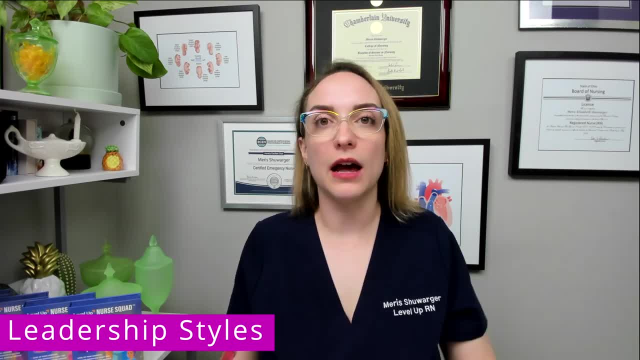 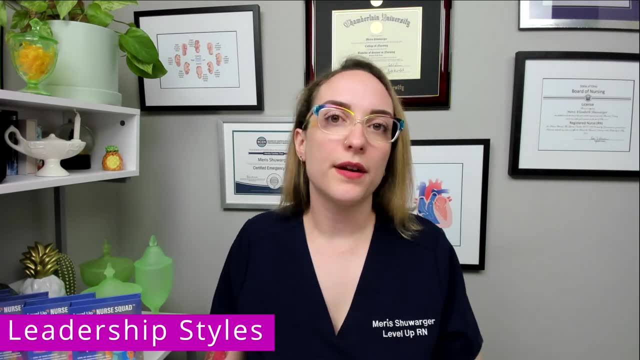 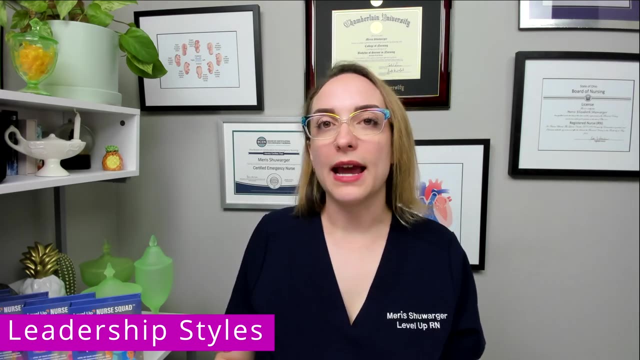 based council where members from the unit of different interdisciplinary team members, the nurses, the techs, the respiratory therapists, you know they all get to have input on what the team is doing and what they see as possible areas for improvement, And then the leader gets to take. 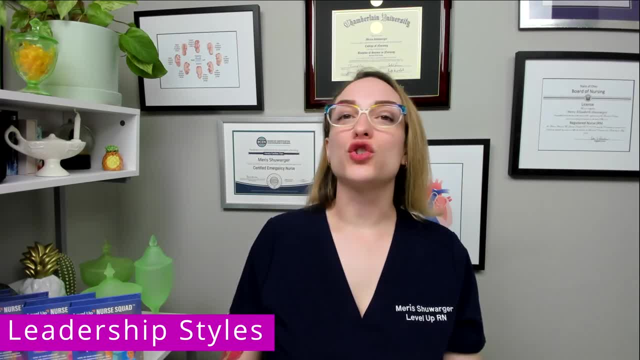 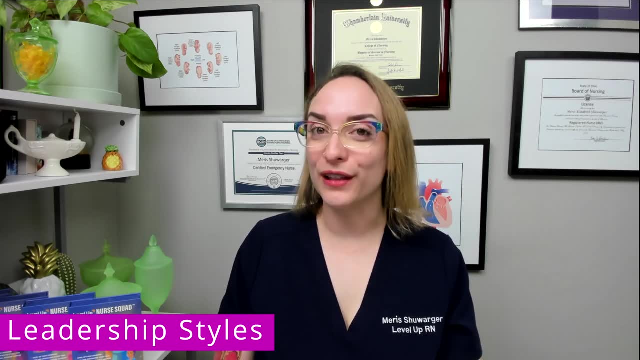 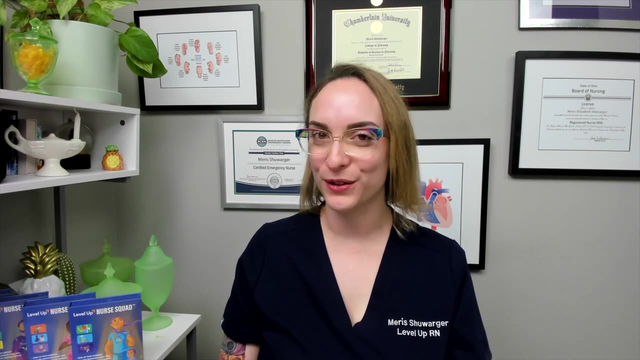 that information and decide what to do with it. We want to transform the culture of the unit to be supportive and caring. Transformational is the ideal leadership style. Okay, That is it for leadership style. I have some quiz questions for you to test your knowledge, So let's see how you. 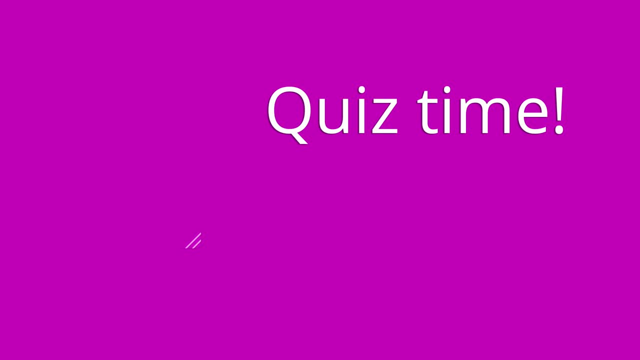 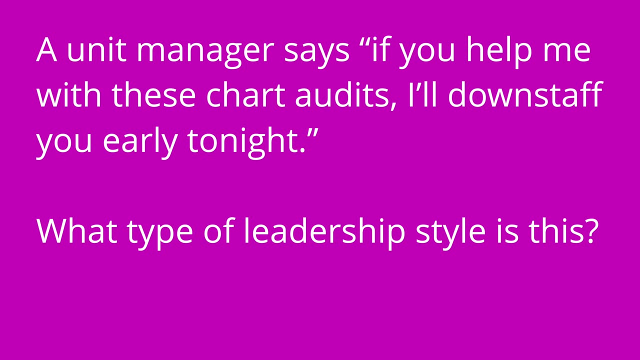 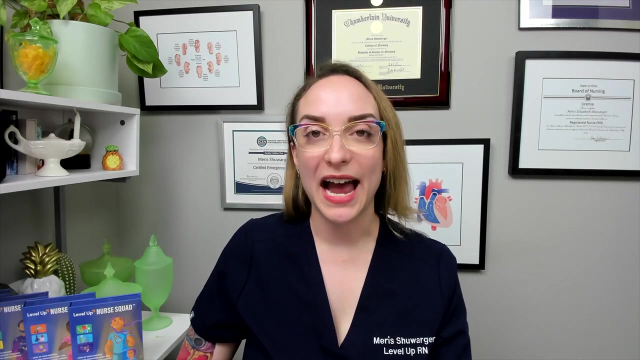 do. Okay, Are you ready to test your knowledge? Here we go. A unit manager says: if you help me with these chart audits, I'll down staff you early tonight. What type of leadership style is this? This is the transactional style of leadership. 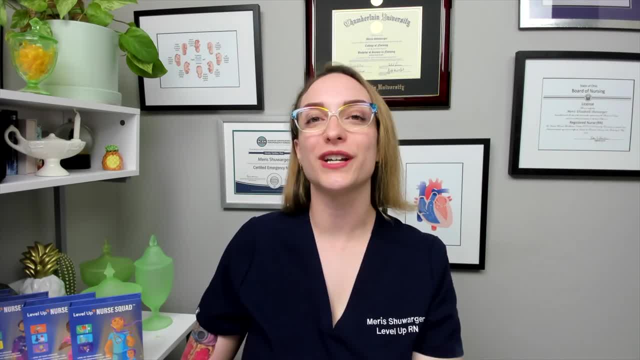 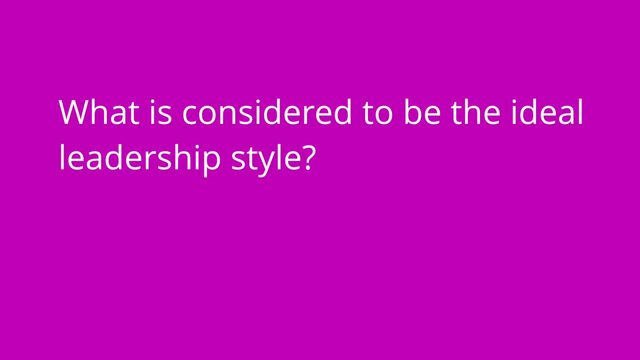 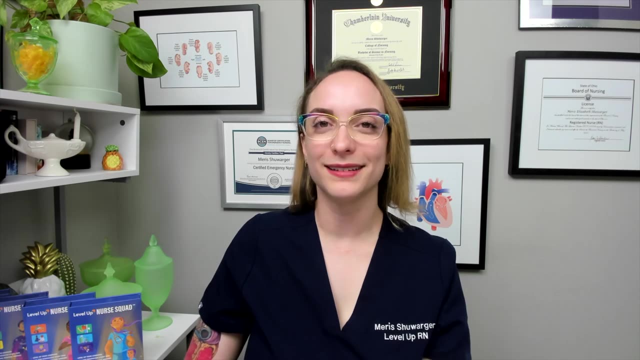 because the manager is providing a reward for finishing a task. What is considered to be the ideal leadership style? Transformational leadership is considered to be the ideal leadership style. All right, That is it for this video. I hope you learned something. Leave me a comment about. 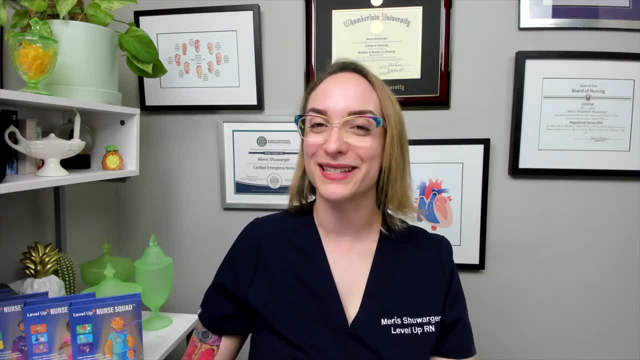 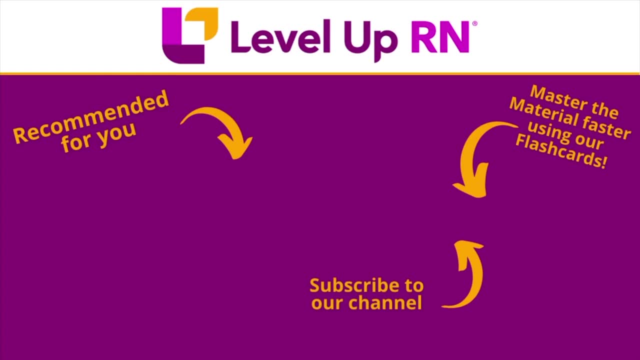 something you learned or experienced about leadership style. I'm excited to hear. Thanks so much and happy studying. I invite you to subscribe to our channel and share a link with your classmates and friends in nursing school. If you found value in this video, be sure to hit.